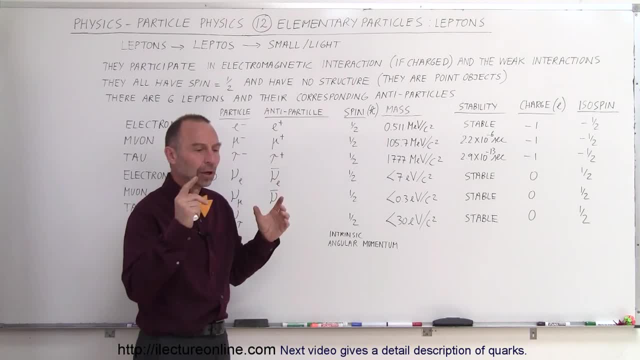 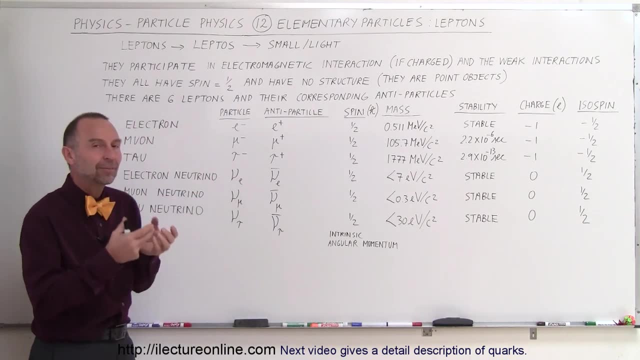 angular momentum spin, Just like in the macro world, objects that are rotating, they have an angular momentum, and so there is a likewise angular momentum existing in the electrons. Now, not that the electrons are spinning just like a top, but it has the same properties as if it was. 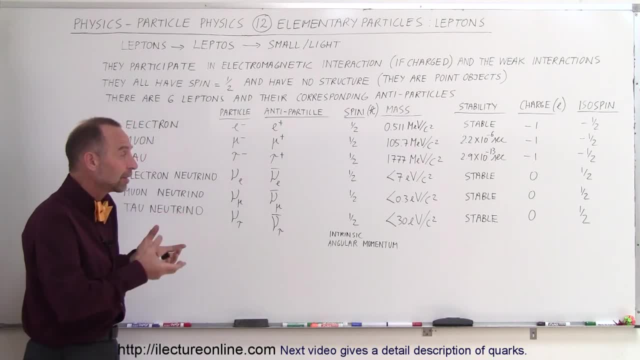 spinning and it turns out that for the electron there's two angular momentum states and it can flip back and forth. So the neutrinos have two angular momentum states and they can flip back and forth between the two, therefore either absorbing or releasing energy from one state to 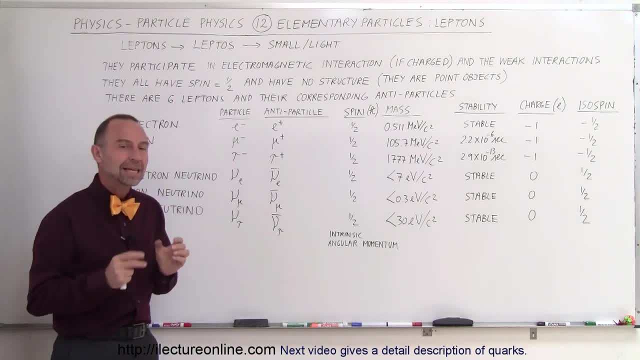 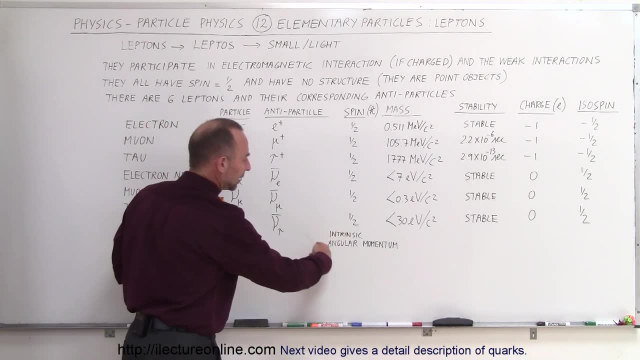 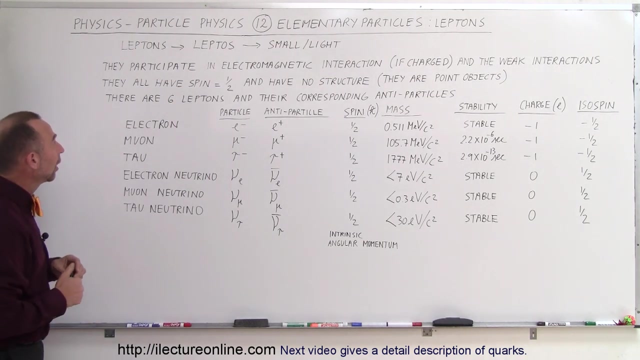 the other when it's inside of an atom, as it's paired up with the nucleus, the positively charged nucleus. So yes, there is indeed something like an angular momentum spin. that's why they call it the intrinsic angular momentum, and the units are h bar, that's Planck's constant divided by 2 pi. What? 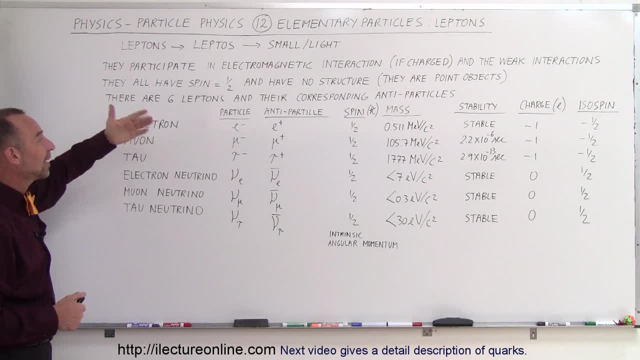 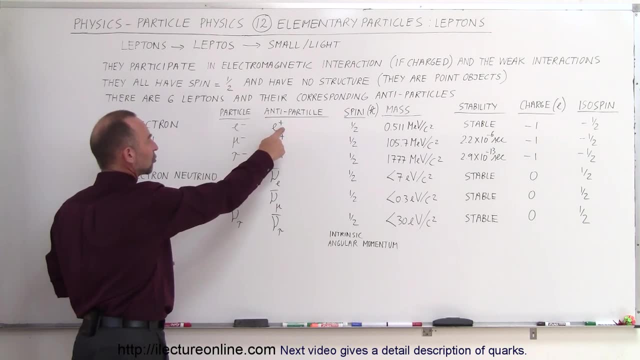 else do we have? So there are the six leptons and they have the corresponding six anti-particles. So for the electron there's an anti-lepton. so for the electron there's a positron, for the muon there's a positive muon, for the tau there's a positive tau, and for each one of the three, three neutrinos. 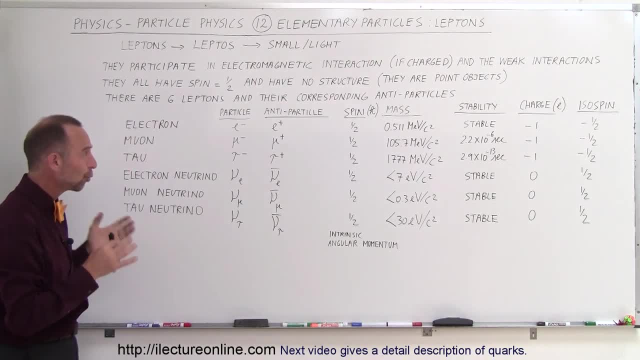 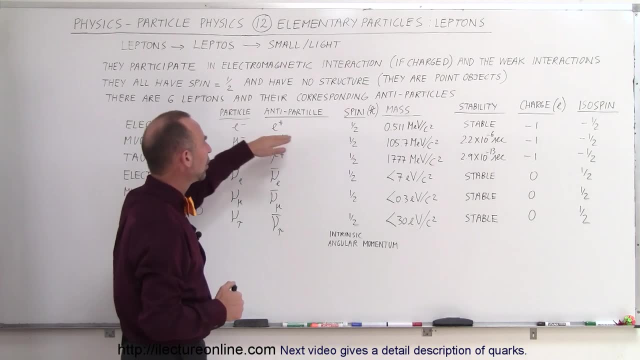 there's an anti-neutrino. So there's a total of 12 leptons: six leptons and six anti-leptons. So let's take a look at their mass. Now, for an electron, you need 511 000 electron volts, or 0.511. 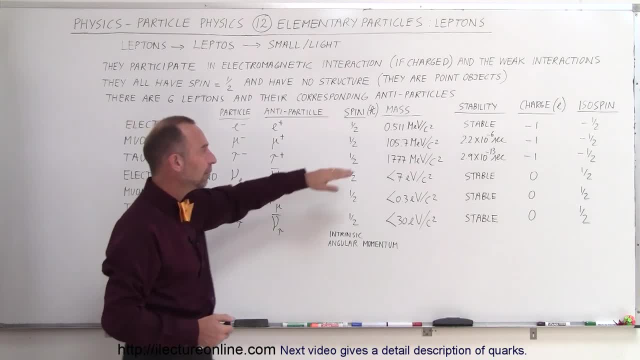 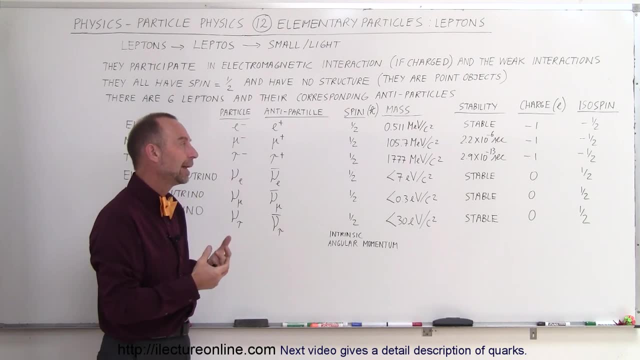 MeVs- M stands for mega or million, so it takes a little bit over a half a million electron volts in order to make to, to have enough energy to make the mass of a single electron. That's relatively small, because the amount of energy you need for a proton or neutron 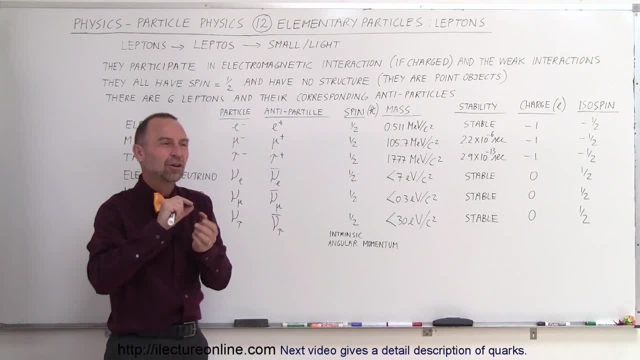 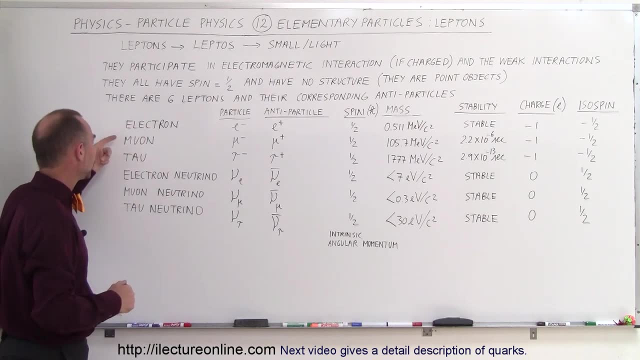 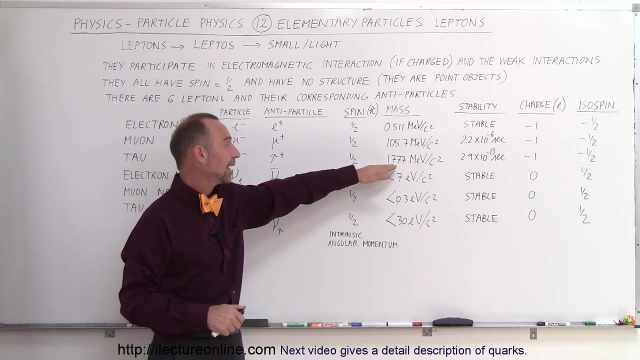 is almost 2 000 times as much. So the mass of an electron is about 1, 2 000 the mass of a proton or the mass of a neutron. Now notice that the other two, the two other particles, muon and tau, they're much larger. This one takes 105.7 million electron volts and this one would take over a. 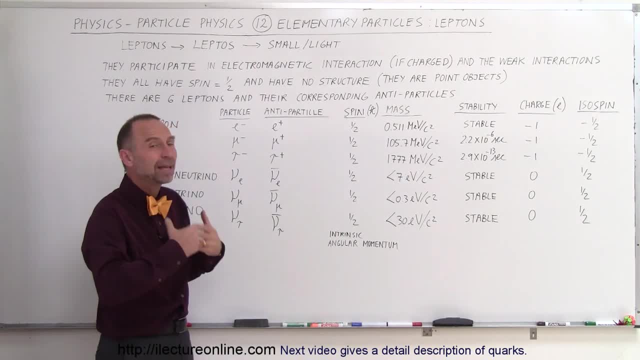 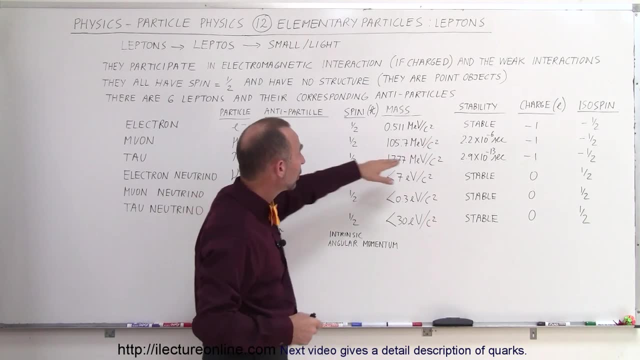 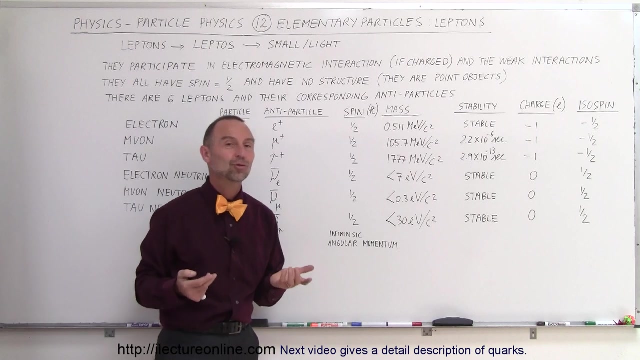 billion electron volts, Or almost 2 billion electron volts of energy, to make that particle. Hence these two particles tend to be very unstable. The muon only lasts for about 2.2 millionths of a second, and here the tau lasts for less than a trillionth of a second before. 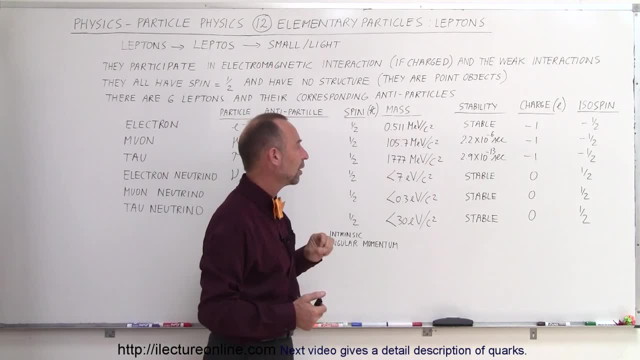 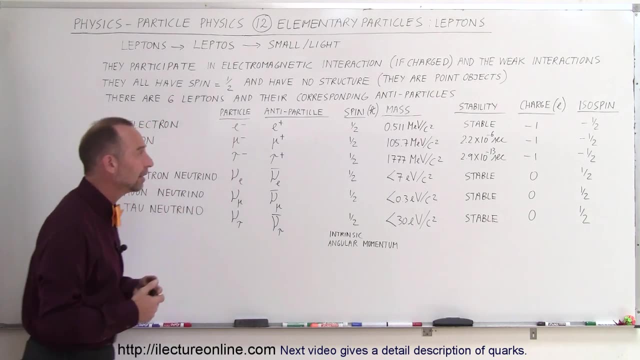 it disintegrates, So these are very unstable particles. They require a lot of energy to create. Now the electron is a very stable particle. It lasts just about forever and therefore it is small and very stable. So are the neutrinos. Now the neutrinos are very strange particles. 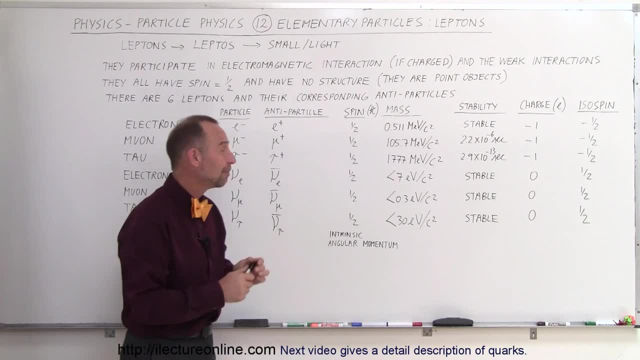 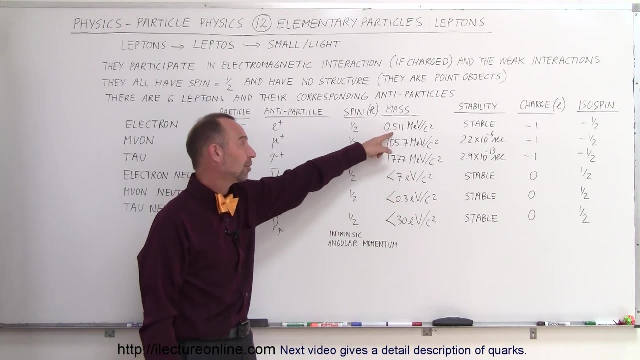 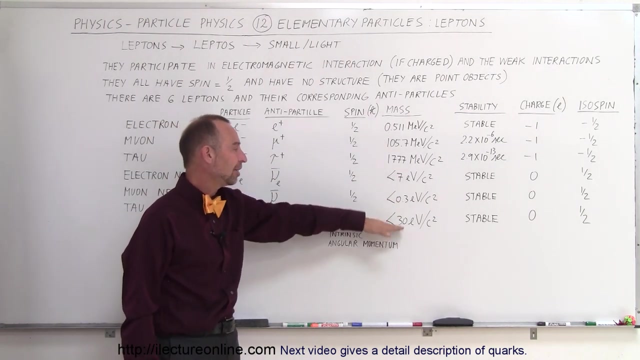 Notice they're extremely small. They have very small amount of mass, Much, much smaller than, for example, electron. In this case it is seven versus half a million, So it's about one in a hundred thousand. So it's about a hundred thousand times smaller than an electron. and these are about a. 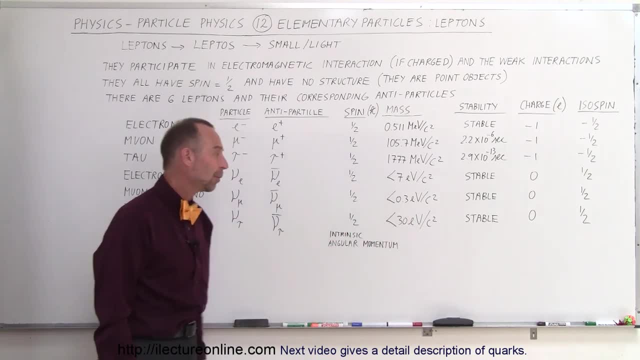 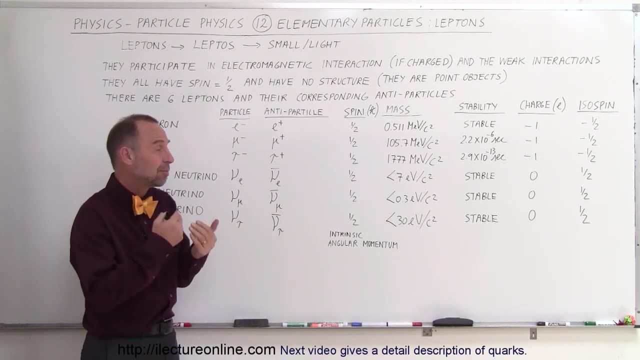 million. This is about a million times smaller and this is about about 150 000 or 120 000 of the mass of an electron. They're still. all three are very small particles and therefore they move at very high speeds, near the speed of light. They used to think that these particles were like photons and 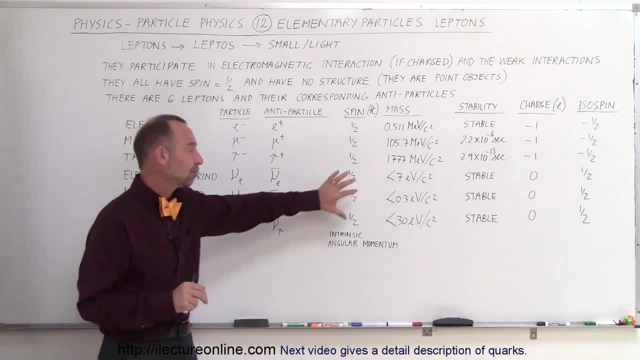 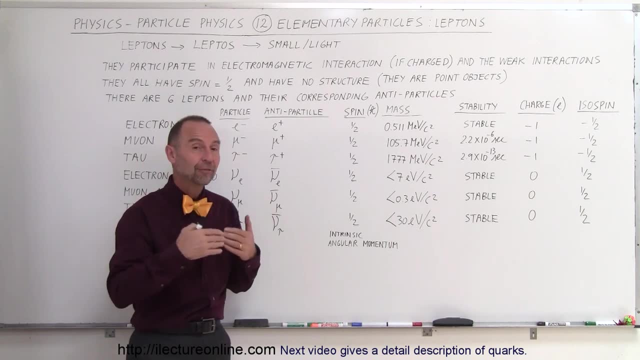 therefore had no mass at all. But now we know that's not the case. They have a small amount of mass, so therefore they don't move quite at the speed of light. Now, what's interesting about it is these particles. they're very elusive. The reason why they're elusive is they carry no charge. 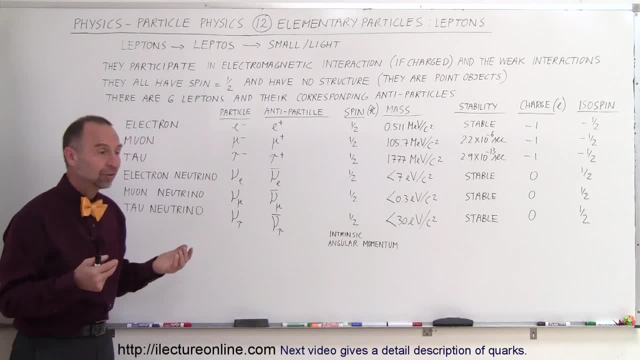 So there's no interaction with the with matter. However, the only way that they can interact is if they actually are in a head-on collision with a particle like a neutron or a proton. Other than that, these particles tend to go straight through just about any material, and these particles, matter of fact, go right through you right now, As you're. 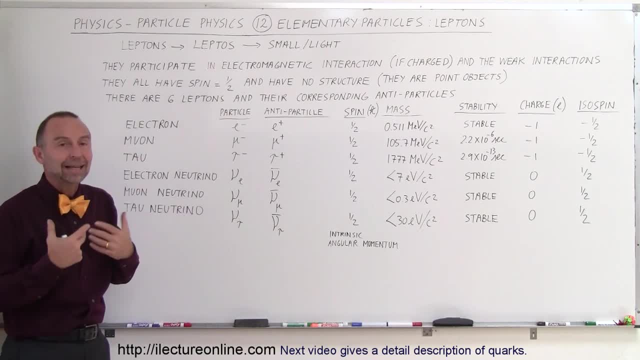 sitting there watching this video. there's neutrinos going through your body and not interacting at all with any atoms in your body and they continue right through the earth and continue to come out the other side of the earth, and most of them do not interact with any matter inside the earth as 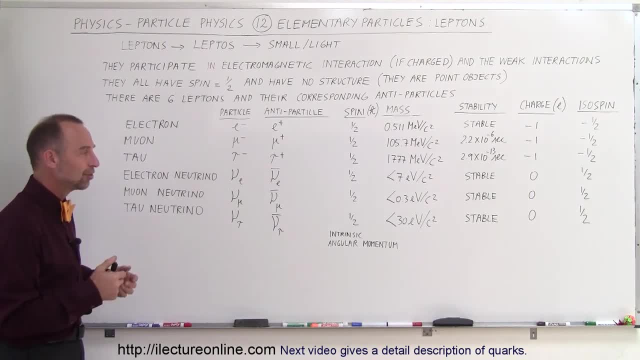 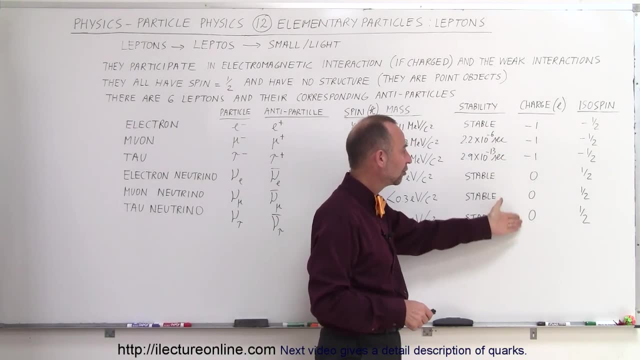 they go right through them. So they're very, very elusive particles, Very strange kind of particles. Let's see here, other than stability, we have the charge- Notice that these have charge, these don't have charge- and they also have an isospin related Here, the 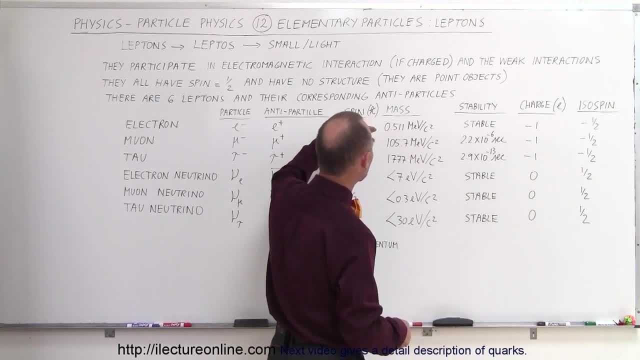 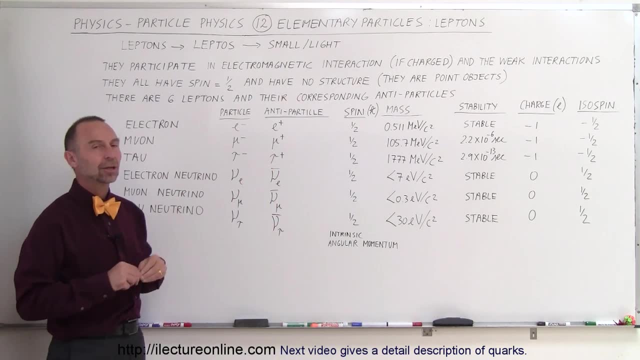 isospin is minus one half for the electron, the tau and the muon, and they're plus one half for the neutrinos. Now, the isospin is a quantum mechanic number that is associated with what we would call the strong interaction, And it turns out, since these leptons do not interact with the